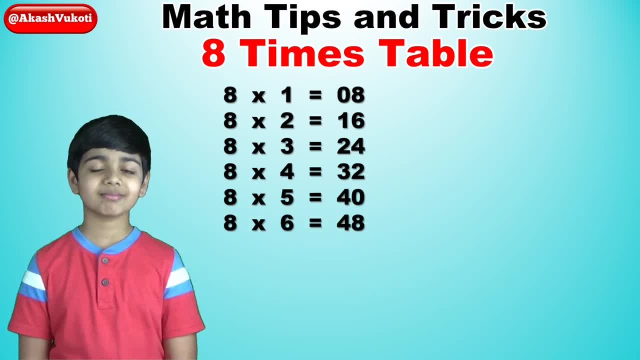 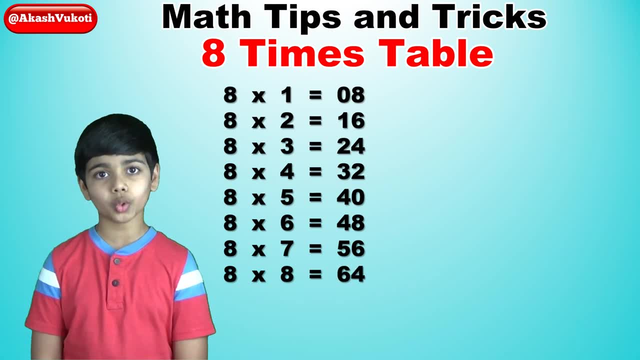 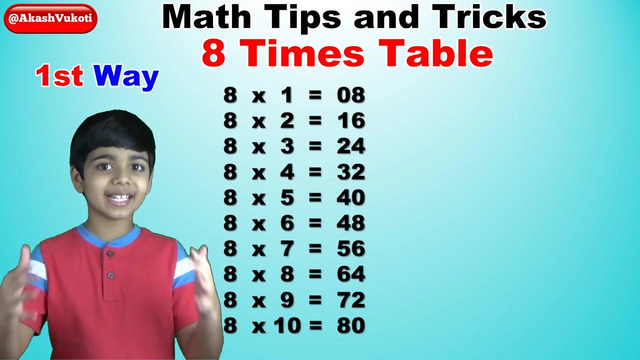 Eight times six is forty-eight. Eight times seven is fifty-six. Eight times eight is sixty. Eight times seven is fifty-six. Eight times eight is sixty-four. Eight times nine is seventy-two. And finally, eight times ten is eighty. Now, here's the first way of explaining the trick, As this is the eight times table. 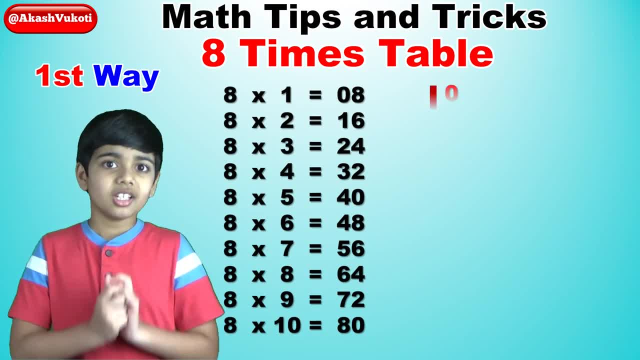 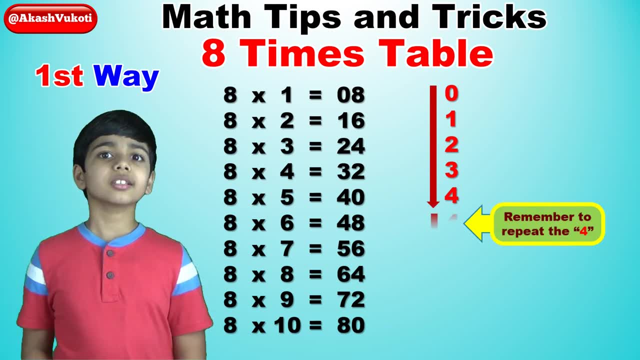 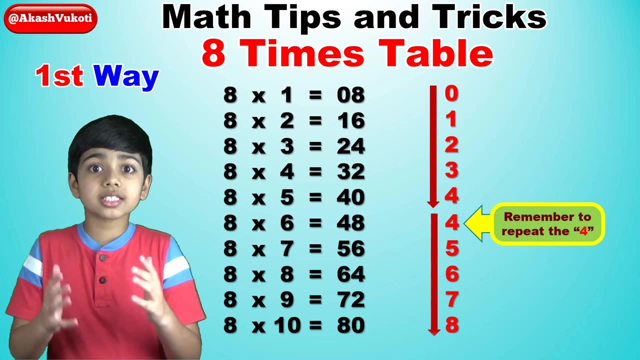 write down all of the numbers, from zero to eight, from top to bottom, as you're seeing behind me right here. But once you reach four, include an extra four and then repeat the same process and your practice will abandoned and continue until eight. 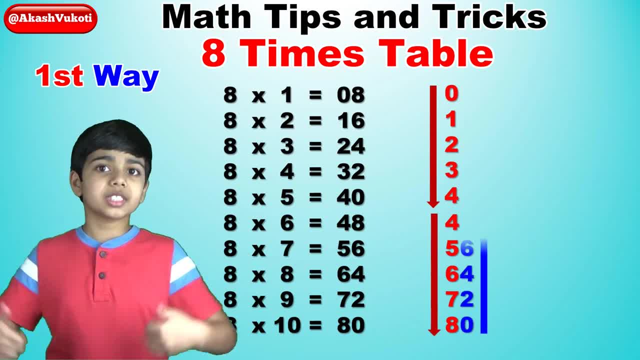 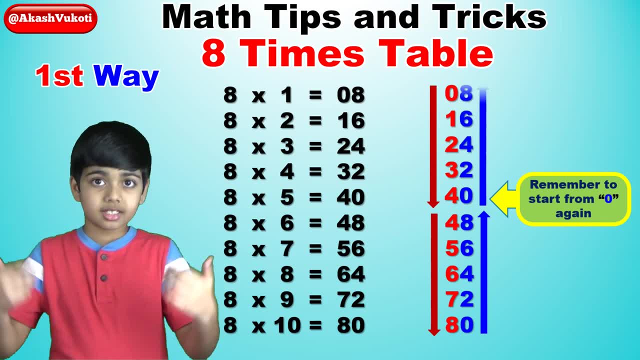 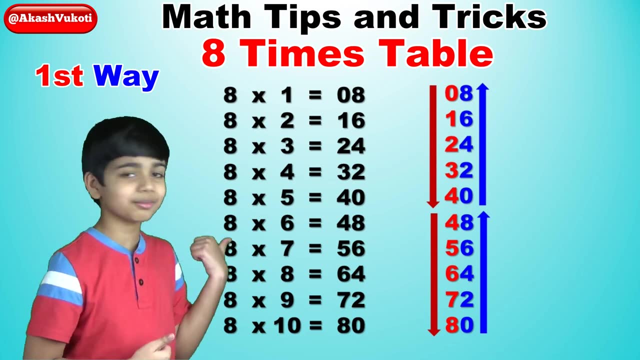 Next, for the ones digits, write the two times table, starting from zero up to eight, again from bottom to top, And once you reach eight, repeat and go again from zero up to eight And once you're done you have the eight times table, as you can see right here. 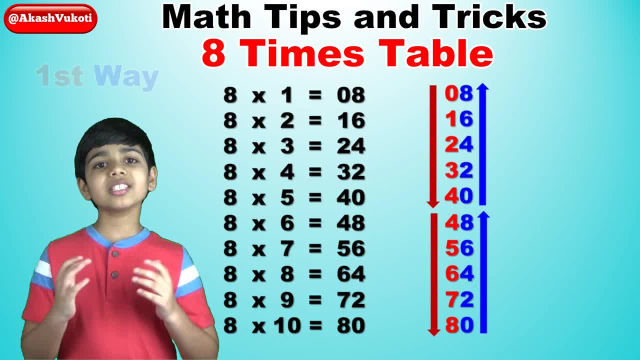 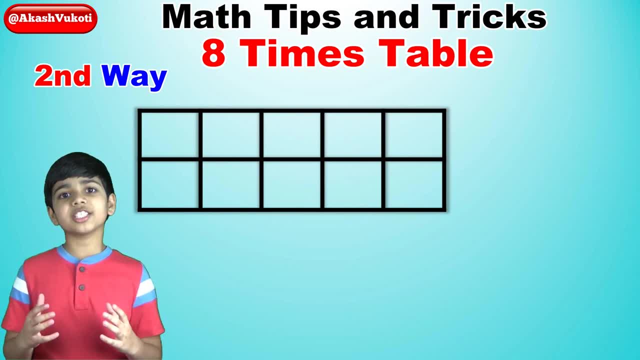 second way of explaining the trick, as you can see here, let's create a box of five columns and two rows for the ones digits. just like you've seen in the first method, we're going to write down the two times table, from 0 to 8 in both. 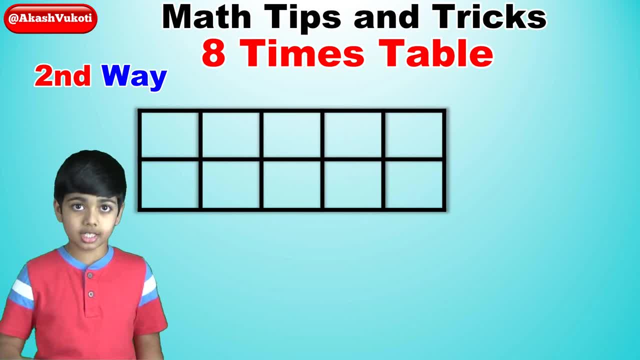 rows, but this time backwards, in the opposite direction, from 8 to 0. so 8, 6, 4, 2, 0. now for the tens digits. in the first row, we will write down the numbers from 0 to 4, as you see here, and for the tens digits in the second row, we will 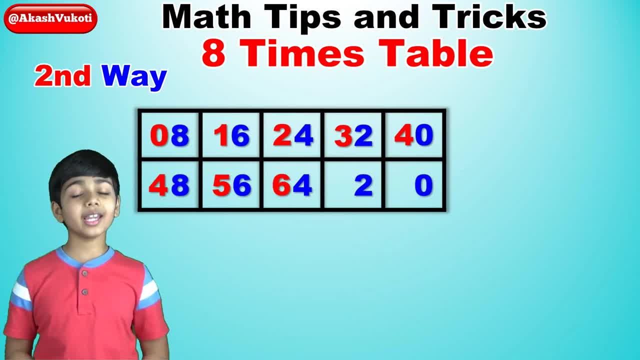 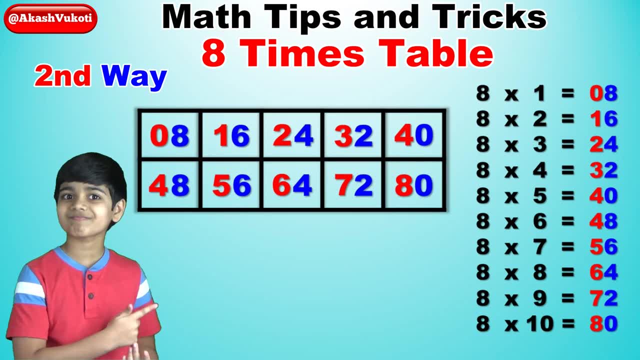 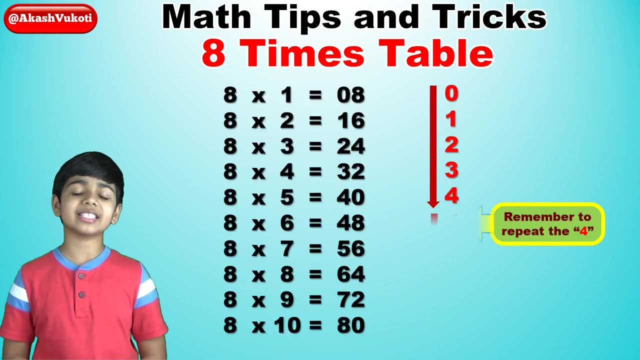 write the numbers from 4 to 8 and once you're finished, you will have the 8 times table, as you can see right here. so now you have seen two, two methods for learning the 8 times table. you can choose one of the methods and. 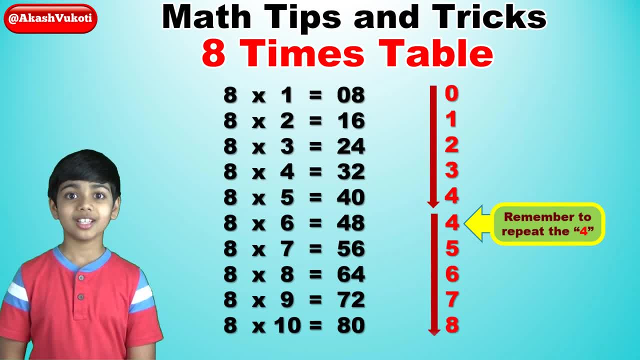 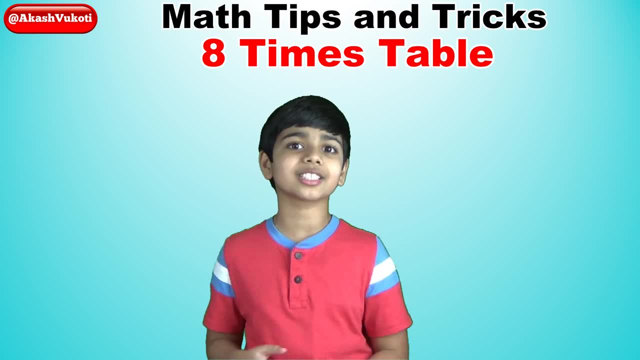 start memorizing the 8 times table, and that's about it. thanks so much for watching this video. if you like my videos, please subscribe to my channel and don't forget to click the bell icon so you don't miss my new videos every time I upload. once again, thanks so much for watching. love you, Akash.